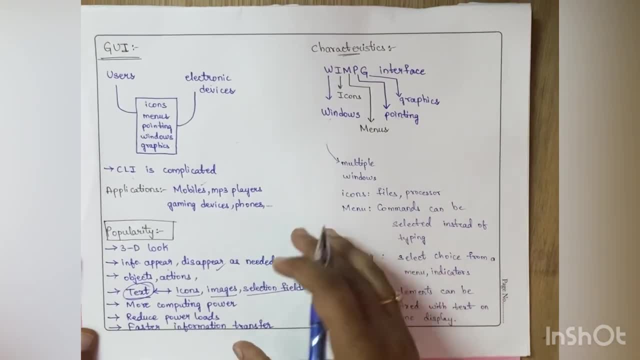 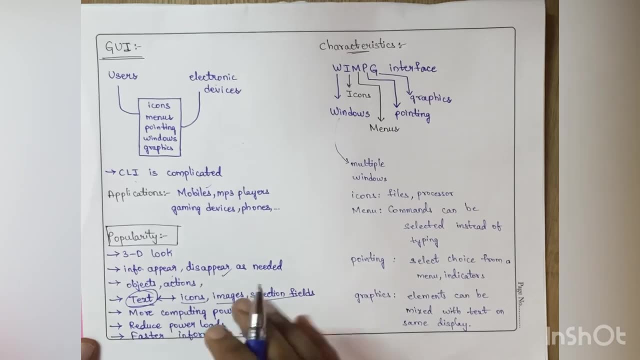 increased because now people, now they are easily attracted for all these images. That means because symbols are very easy to remember than the commands right. So because of that the computing power increases and it also reduces the power loads and the faster information transfer. 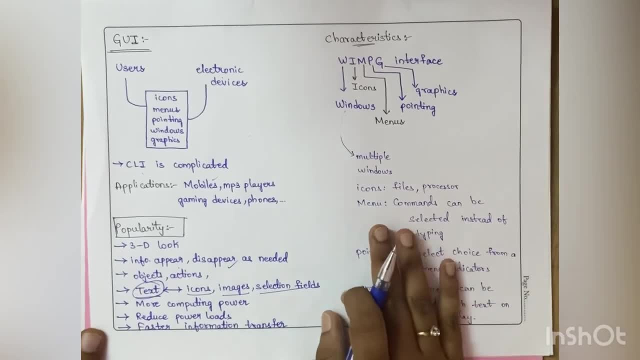 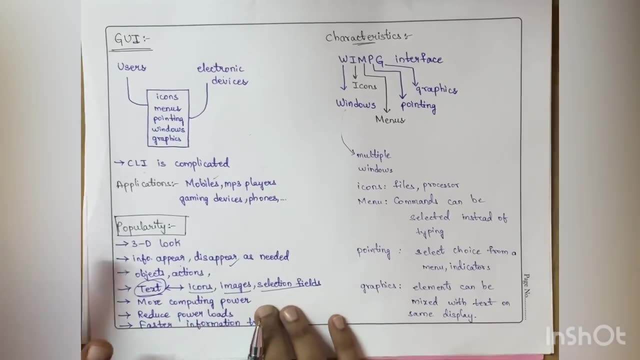 That means between two computers we can transfer any information very securely and fastly And this is the popularity of GUI. And there are many things in the list of this popularity. I have mentioned a few things here like 3D, three-dimensional- look like information. 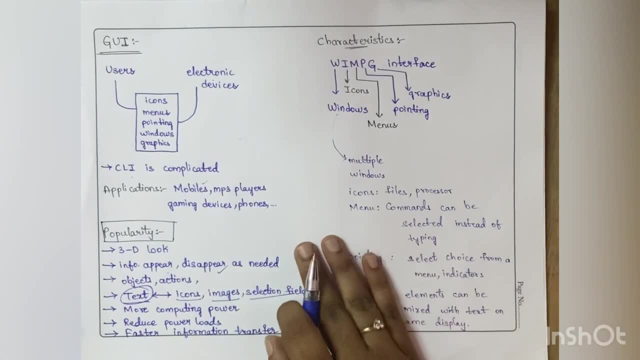 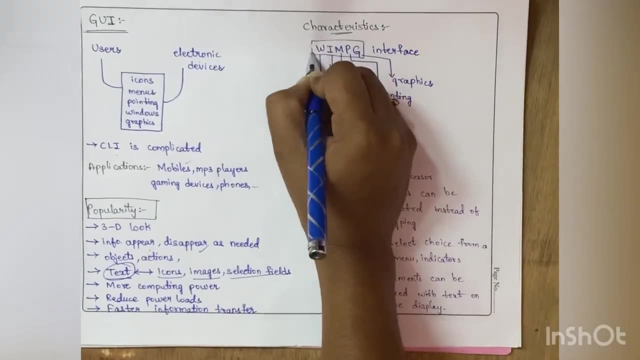 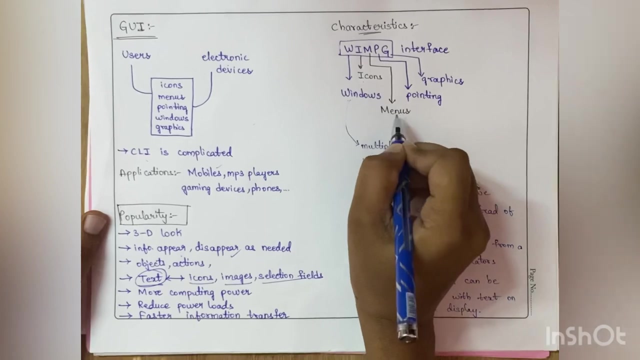 appear and disappear. So all these things, And you can also learn many other points from the Google. And coming to characteristics, So if you remember this WMPG interface thing, you can write all the five characteristics That means here. WMPG is like windows icons. 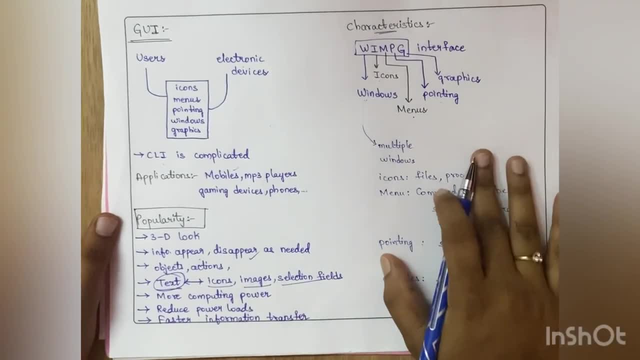 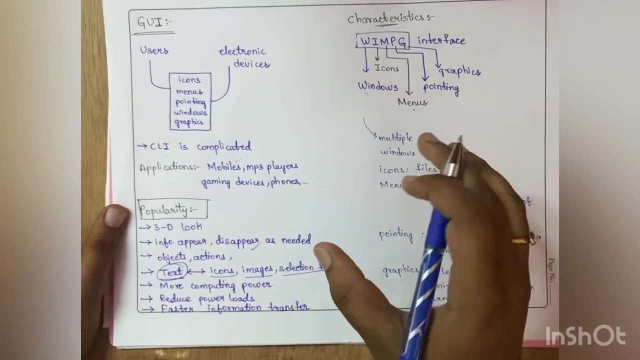 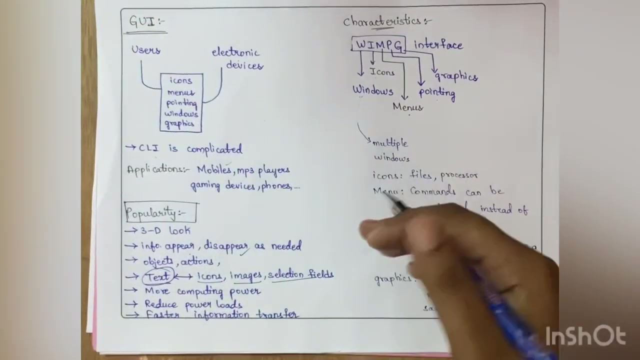 pointing and graphics. So what is this windows Like, say? suppose like in a laptop, at a time, simultaneously you can watch a YouTube video and you can also study a PDF. That means, like multiple windows can be opened. That means GUI is supporting multiple windows And coming. 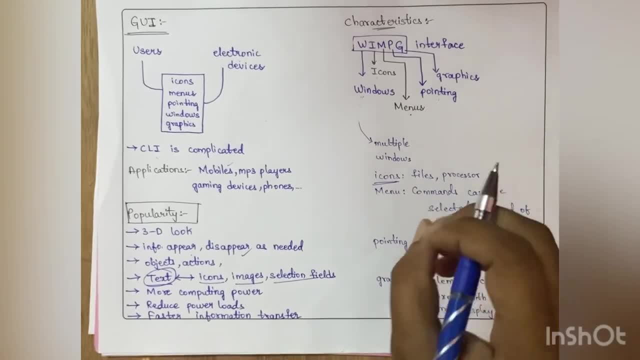 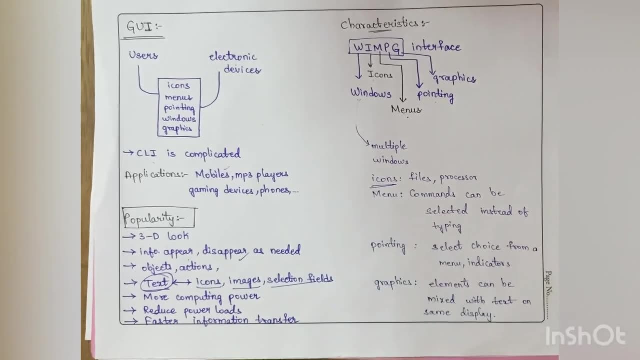 to icons, say, suppose, like we can drag a file. That means files, processes, folders, all these things comes under icons. And coming to menu, like previously, we used to type all the commands. right Now, instead of typing the commands, we can just select the commands. 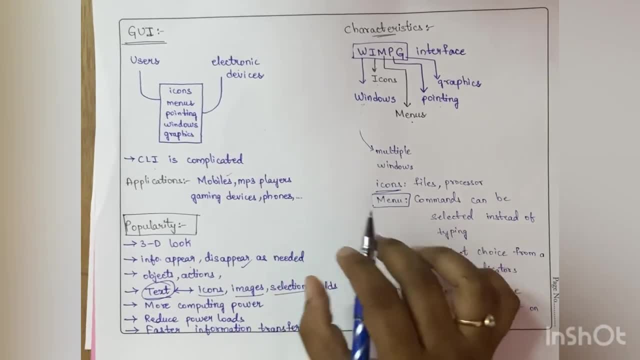 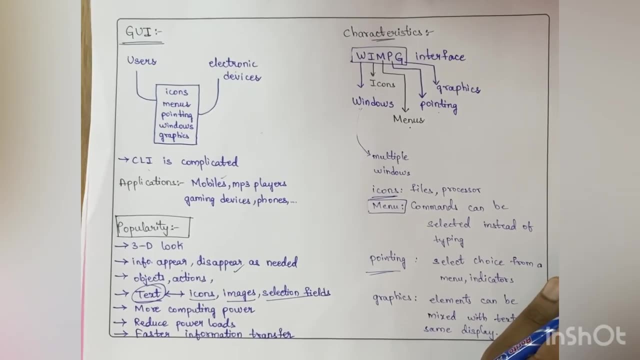 That's it. That means using the menu things. we can just simply select the command. And coming to the pointing things, pointing is like you like. whatever it is necessary for you, you can select from the information which has appeared on the screen. That means selecting choices of your. 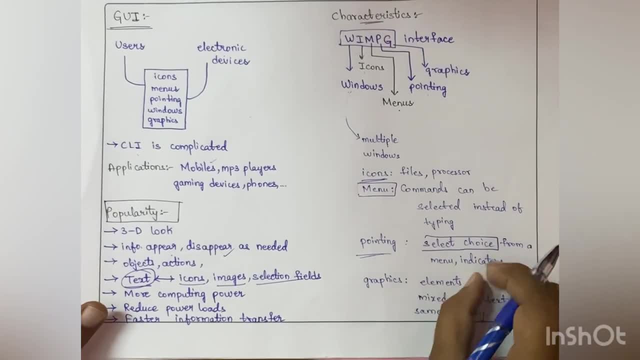 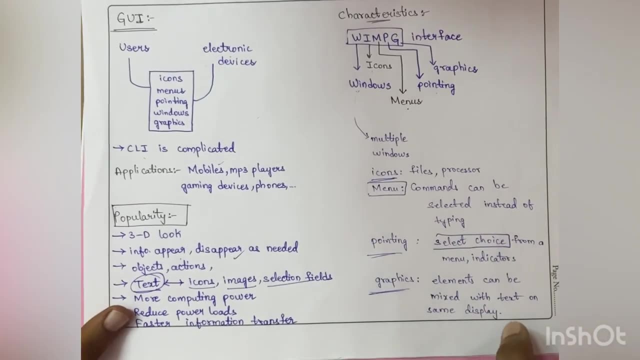 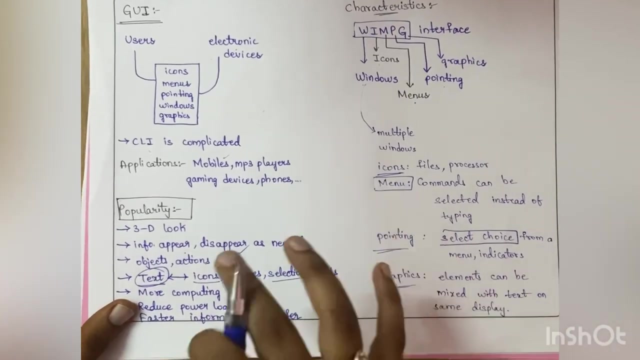 I mean selecting things of your choice using the indicators. Pointing like a mouse comes under the screen right, So that means you can find text along with some animations, some images, all these things. That means hope. you all know like you play many games and all right. So that comes under graphics.